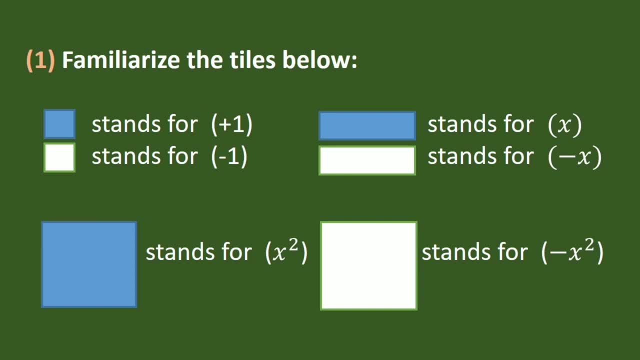 let us familiarize the tiles below: blue square tile stands for positive: 1. negative square tile stands for negative: 1. blue rectangle tile stands for positive: X. white white rectangle tile stands for negative: X. big blue square tile stands for x- squared. and big white square tile stands for: 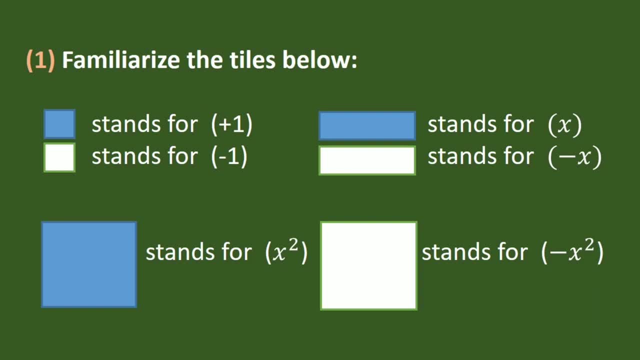 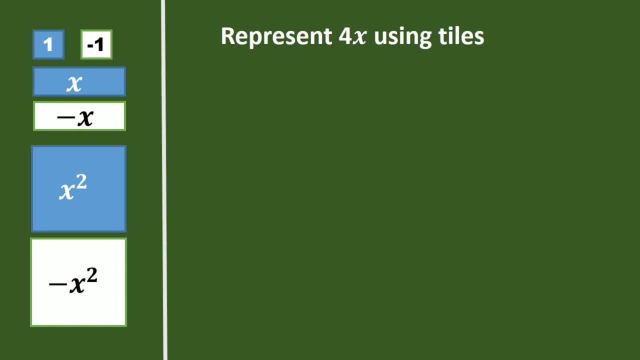 negative x squared, so we will be using this in our operation. represent 4x using tiles. 4x: that means there will be 4 positive X tiles we have. that's it represent 3x squared using tiles. there will be 3x squared tiles: 1, 2, 3, so that's. 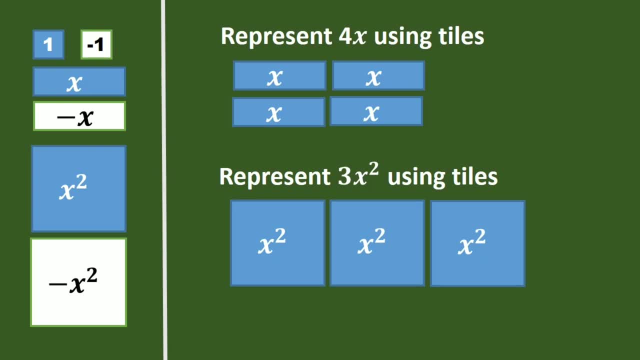 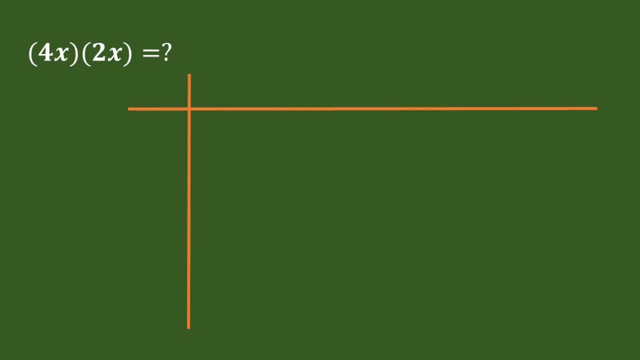 3 X squared. now let's do the operation. for example, we have 4 X times 2x to get the product using the tiles. the less first drew perpendicular segments at the top of the horizontal line or segment. we have 4x and there will be 4 positive X. 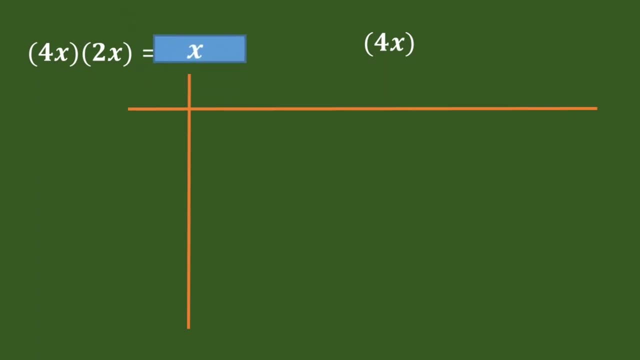 tiles. we write for the put here. that's it. and to the left side we put two X. we have two positive X tiles. So to multiply these tiles, we multiply tile by tile. so we have X times positive X. the answer is X is squared. another X times positive X answer is X. 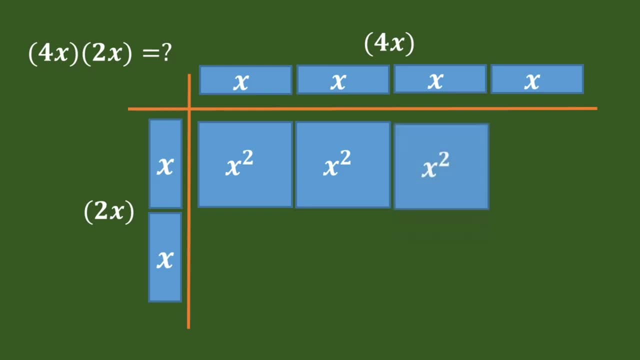 is squared X times positive X. answer is: X is squared X times positive X. the answer is: X is squared. We now have the product in the first row and let's proceed to the second row. we now multiply X times X. what's X squared X times X? X squared X times X. X squared X. 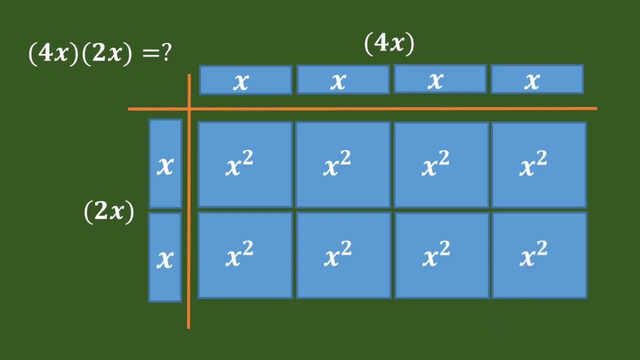 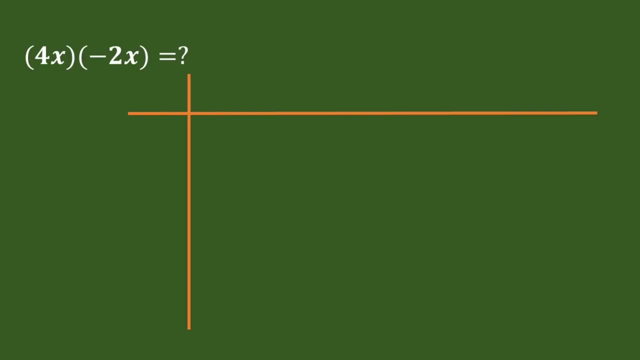 times X, X's. so we are done in multiplying the Pines. inside is our product. so we have to count the piles that are the same: one, two, three, five, six, seven, eight. so we have 8 X squared tiles. our product now is 8 X squared. now let's have an example with the positive and negative factors: 4x. 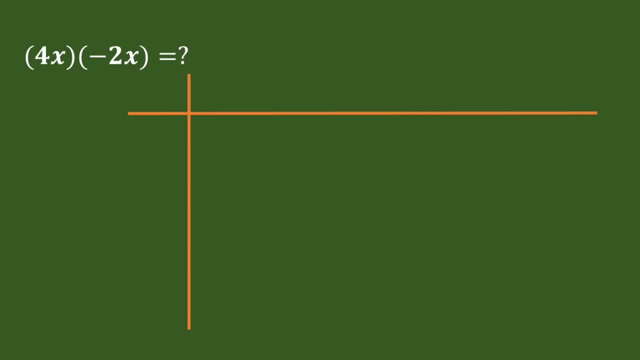 times negative 2x by using the tiles. we have to write above 4x and put the tiles. positive X tiles, four of them, and to the left side we have negative X tiles. there are two, so we multiplied this. I mean negative X is negative x. 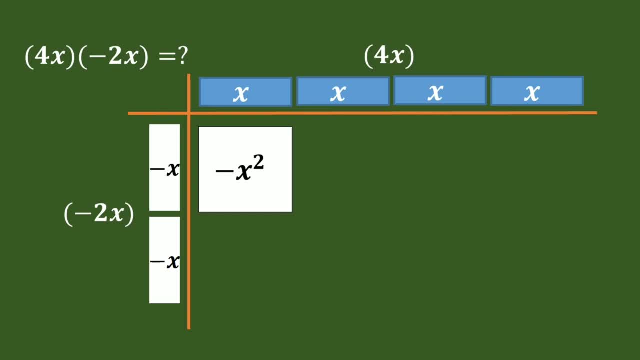 squared, we have the Y square time: X times negative X is negative x. squared X times negative x is negative x. squared X times negative X is negative x. x is what we are done with the first row, so let's proceed for the second row. so X times negative X is equal to negative X. square X times negative X is negative X. 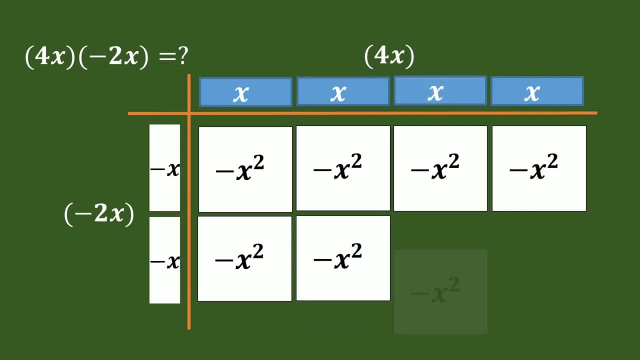 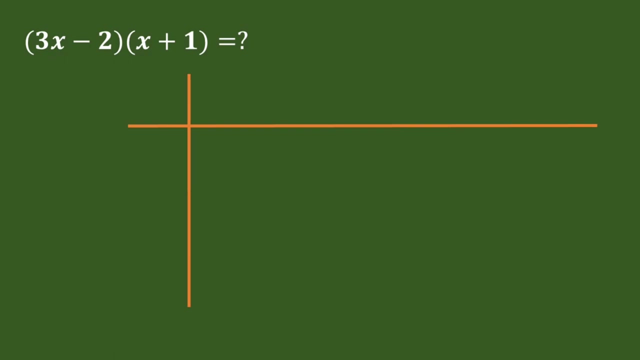 squared X times negative. X is negative, X squared X times negative. X is negative, X squared. so our product is placed inside the soul. let's count the negative x squared times, and there are eight. so our product is negative: 8 x squared. another example: we have two binomials. we will get the product of this: 3x negative, 2. 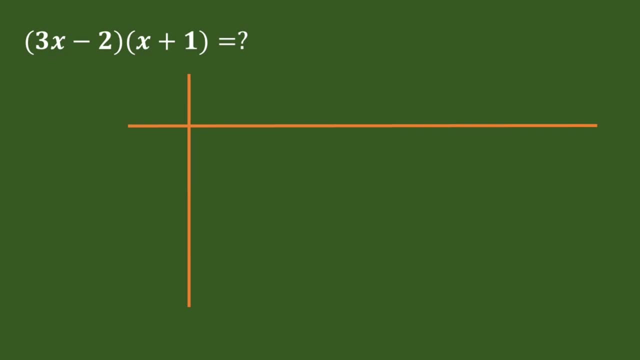 times X positive 1. get the product using the tiles we have. we have 3 positive X tiles. for negative 2 we have negative 1 tune. you have 2 negative 1 times and X positive 1. write it on the left side. we have 1 positive X tile and 1 positive 1 tile. X times positive X is X. 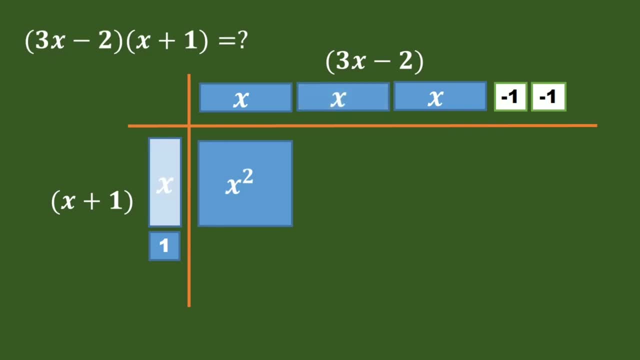 squared: X times positive X is X squared and X times positive X is X squared. then we have negative: 1 times X is negative X. another 1 times X is negative X. so we are done with the first row. let's proceed for the second row. so X times positive: 1 is X. X times positive: 1 is X. 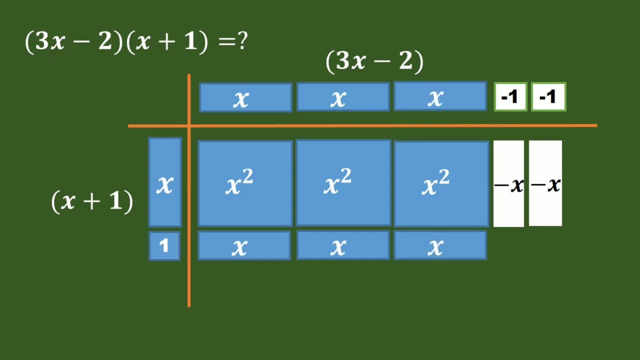 X times positive, 1 is X. so we have 3 X tiles and it's proceed with negative 1. negative 1 times positive is negative 1. negative 1 times positive, 1 is negative 1. so we are done multiplying both sides. so our product is here in the middle. so notice, we have negative X and positive X.